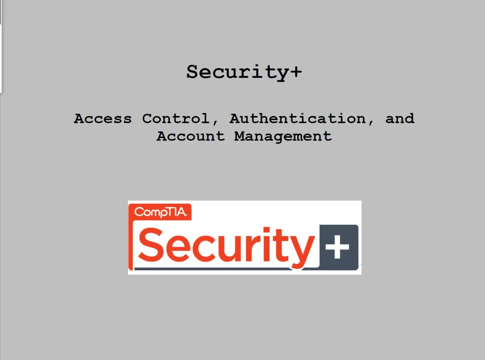 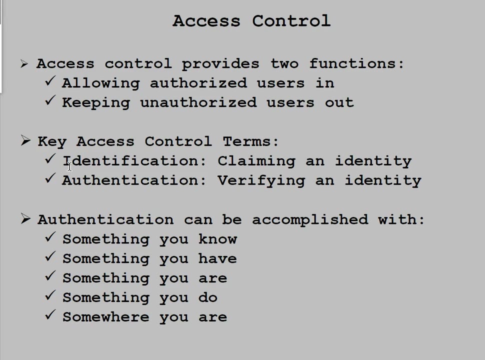 How do we allow somebody in or prevent somebody from accessing through access control? right, We'll talk about kind of the details of that and how it winds up playing into the things we're talking about here. I actually have a bigger section on that in the cryptography piece, Yeah so, but what we can talk about is: you know the process, because as we move forward, 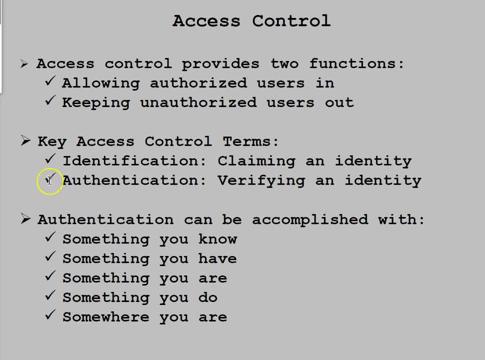 there's actually a very robust section in there on cryptography for PKI. Okay, so most people are probably familiar with the concept of having a couple of different methods of access control. The ones that you should be automatically familiar with is this concept of identification versus, you know, authentication to a system, right? 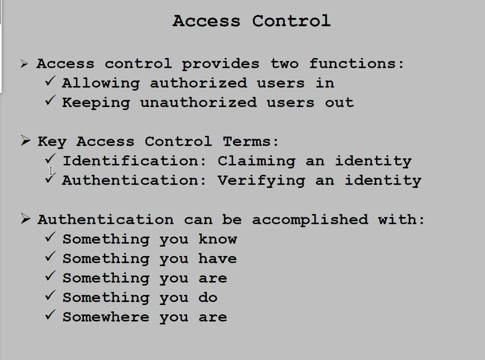 And identification is just trying to state: hey, I am Person X, Okay, this is who I am. Well, how do you prove that right? And this is kind of where the authentication piece comes in, because now you're kind of verifying that you are who you say you are. 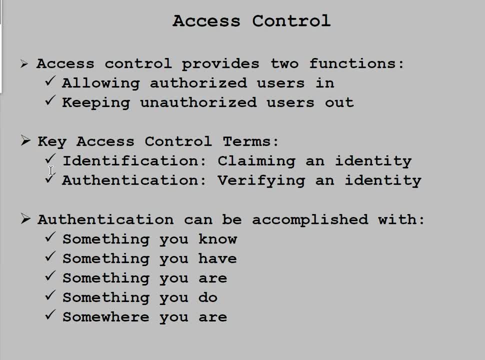 So there's a couple of different ways in which we can do that. You can either have something that you know, right, So what would be an example of something that we know as far as from an authentication standpoint? All right, so a PIN number, password. you know something that needs. 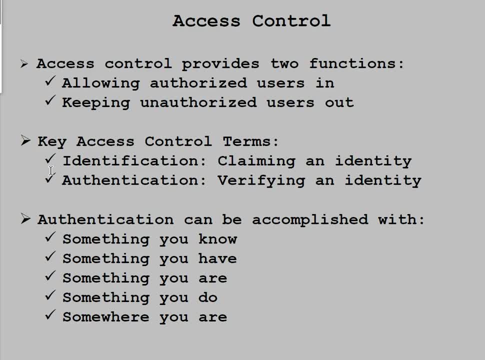 To be, you know, memorized in order to do that something you have, so, on smart card, PKI, being able to go through that process, Maybe you have a, you know, a key fob or something like that that goes in that you have access to, and or, lastly, something that you are. 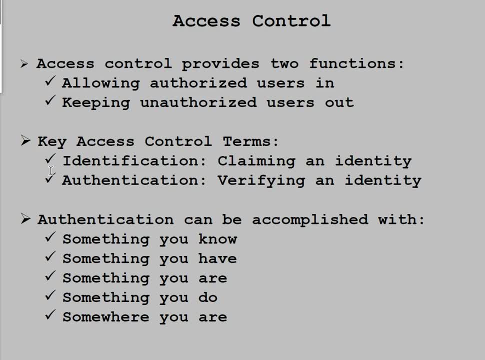 Right, So from a standpoint, what would be some examples of that? Okay, yeah, so anything where you have a ability to be able to prove yourself through your- you know- own individual characteristics and be able to do that as well. 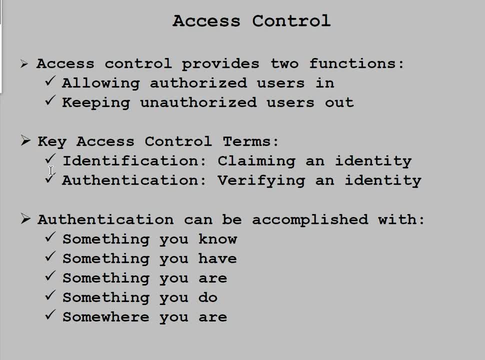 There's other. there's also some other types of technologies that are currently in development where, based on your job, like what it is that you do, you know being able to prove out who that is or somewhere that you are, But both of 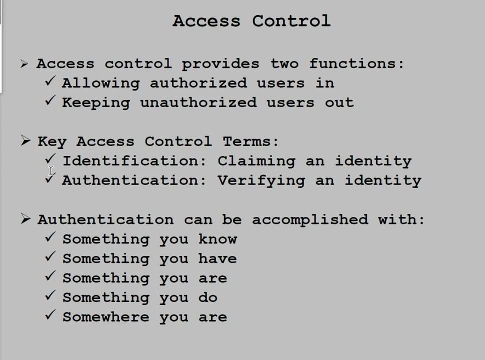 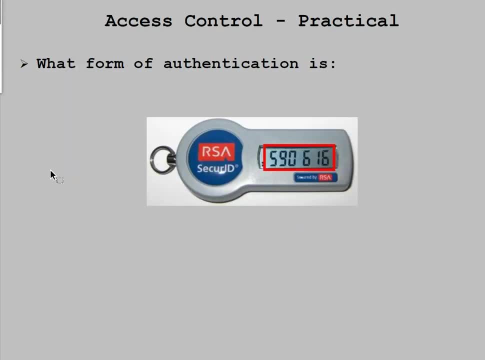 The. Those are a little bit more prone to spoofing and some, you know, modification, so they're still kind of work in development right now. so let's start with a little bit of a practical exercise. so out of the forms of authentication that we talked about already, which one would this be okay? so 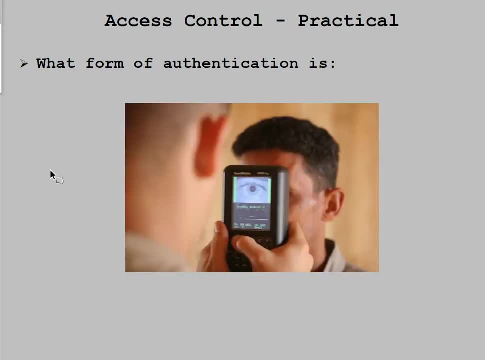 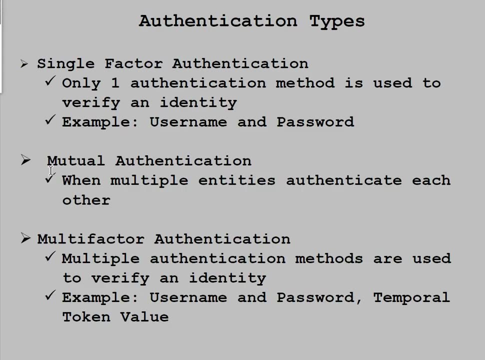 this is something that you have makes sense, right? okay, how about this one? all right, something that you are, and then a couple of different things to keep in mind when we're talking about authentication- is the different methods of authentication can be helped or aided by having you know, maybe more than one. 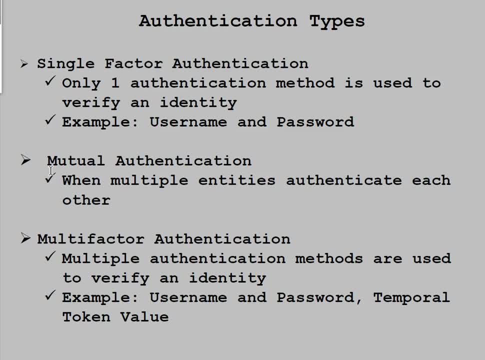 so in the case for a single factor, where maybe you're logging in just to your gmail account and you're just using a password you know, the single factor. authentication is only as strong as somebody not knowing your password if they're able to go through and do a brute-force attack or if they're able to collect. 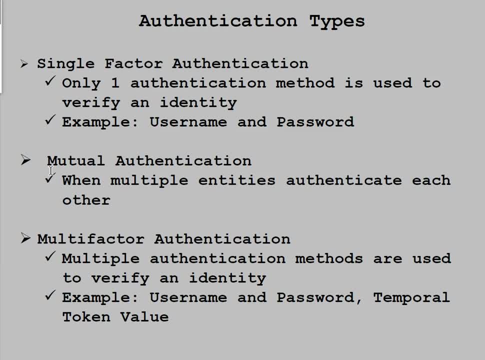 information about you that lends itself to finding out your password. that could be at risk. so what winds up happening is you can have what's called multi-factor authentication, where you go through and now you have multiple methods of being able to identify who you are. okay, and this could be, you know, username tokens. 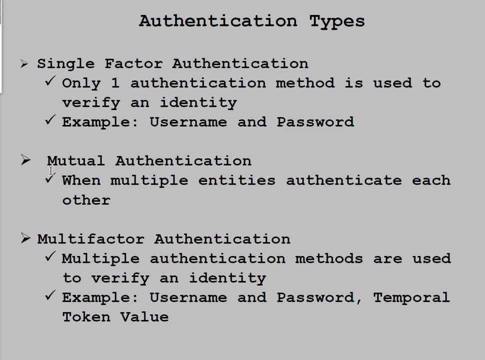 and so forth that most people are familiar with. and then, finally, we have this concept of mutual authentication, where you essentially authenticate to a server and the server authenticates back to you, so both users are have an authentication mechanism going on. alright, so, between our single factor and multi-factor, 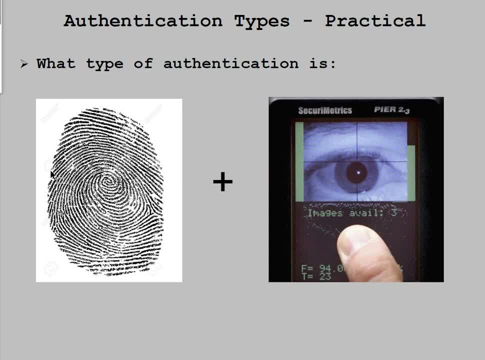 authentication. what would this be an example of this? first one, very good. so, recognizing that, just because you provide multiple methods of authentication, if they're not in the different classification, it's still only a single factor: authentication. you know, now, in this particular case, this would be a pretty strong one, because it is, it is your, you know your biometrics, which